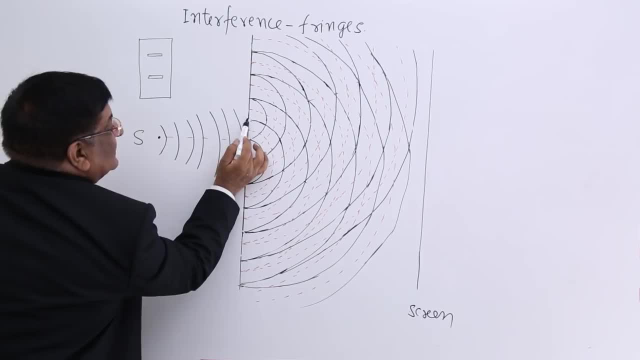 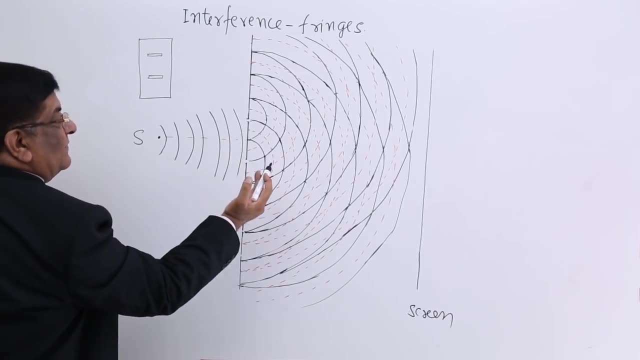 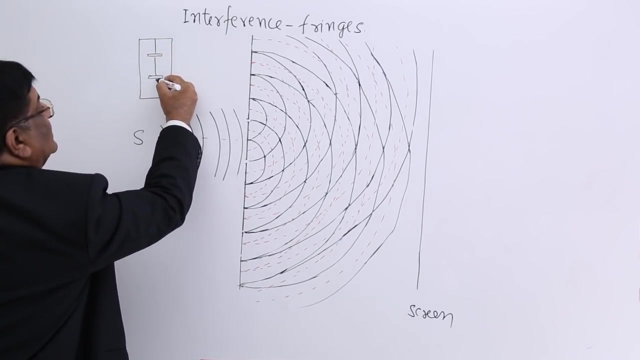 So these 2 openings- one is here and one is here, A wavefront, this or the next or the, any one strikes this, This wavefront portion, This portion, this portion is blocked by the card, but the point here become independent source and start. 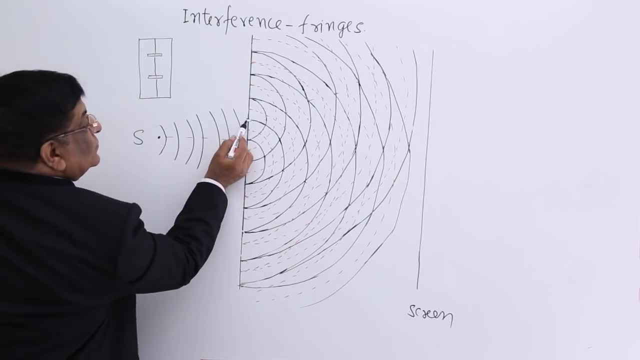 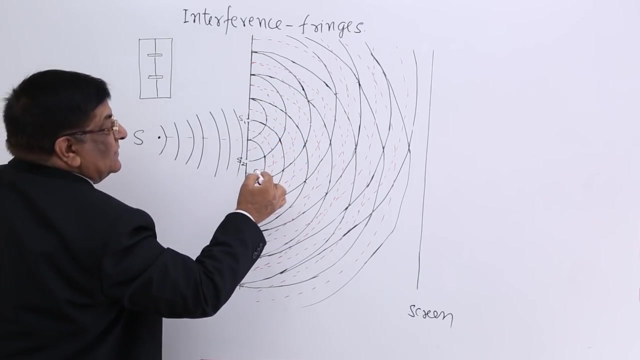 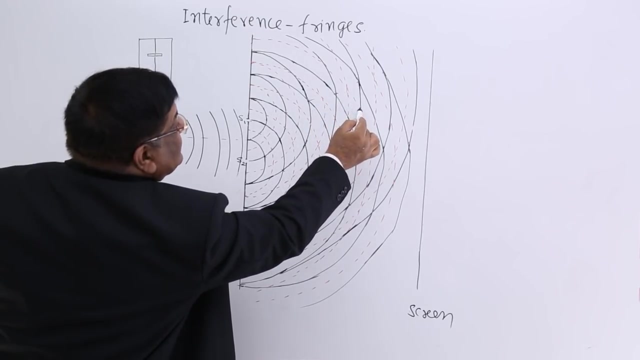 sending its own waves. This is source S1,. this is source S2.. This source S1 start sending its wave. See, I have represented by this is a crest trough red, one crest trough red, one crest black trough red, crest trough crest trough crest trough crest, and the wave goes on. 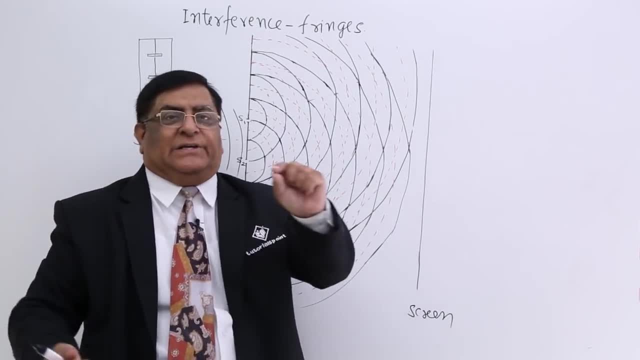 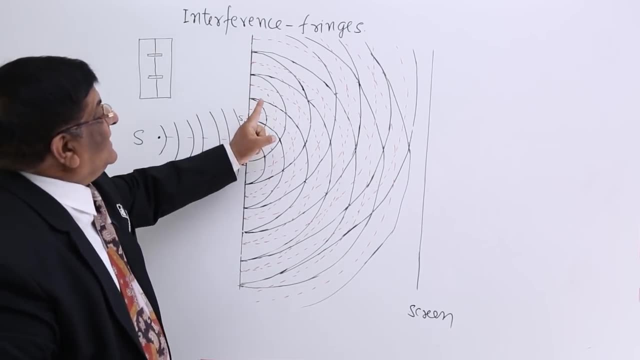 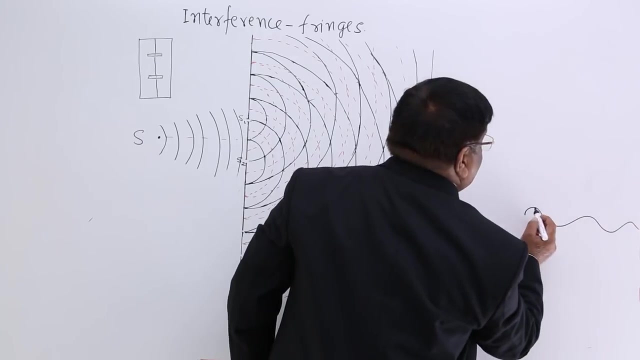 In which direction? In all the direction, Because it is just like a plane. This will go in circular manner. So this is crest trough, crest trough, crest trough. I can say that this is in this shape. If I see it from the side, it will be like this: 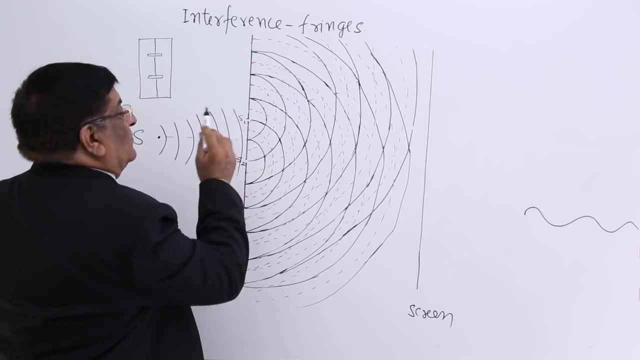 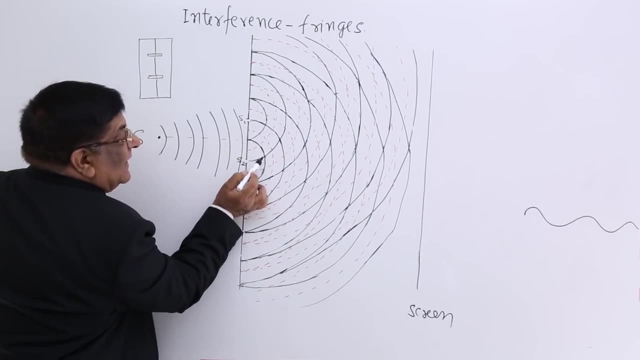 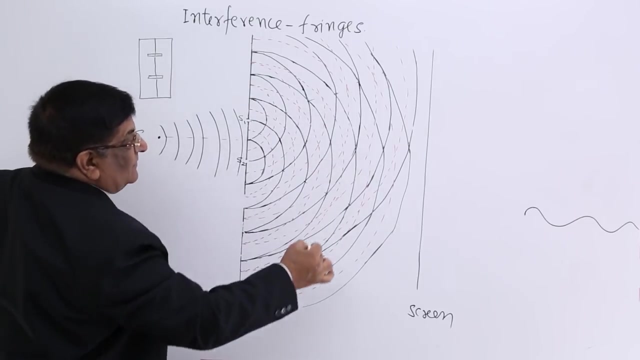 If I see it from the top, it will be like this: That is from source 1.. Now see source 2.. Source 2 has made this crest and this trough This crest, this trough this crest, this trough this crest about this, it has made its own. 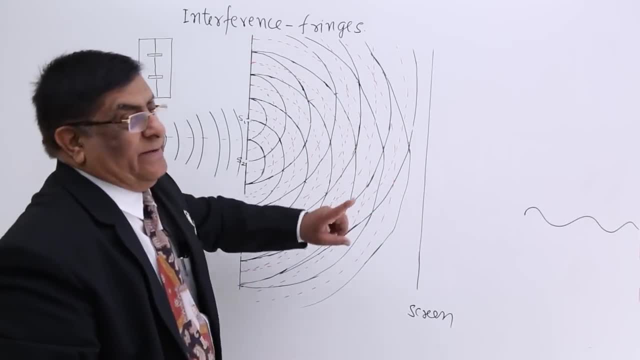 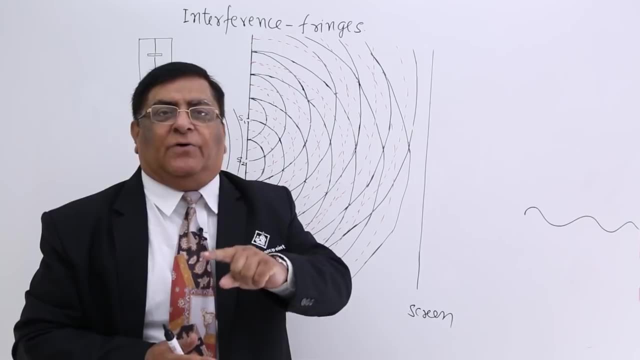 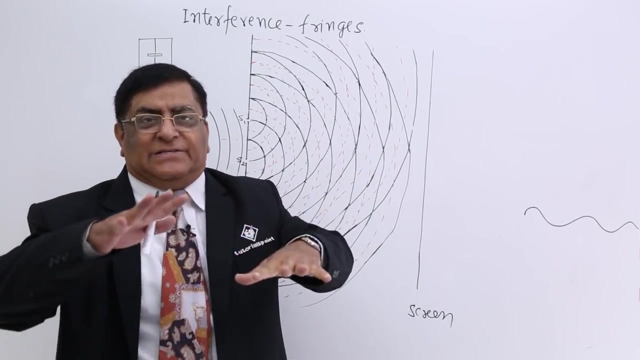 crest and troughs like this. Now, medium is 1.. If medium is 1, both are sending their energy in the form of waves. that is disturbance of the light here, and that disturbance is in the same medium. So this is a wave. 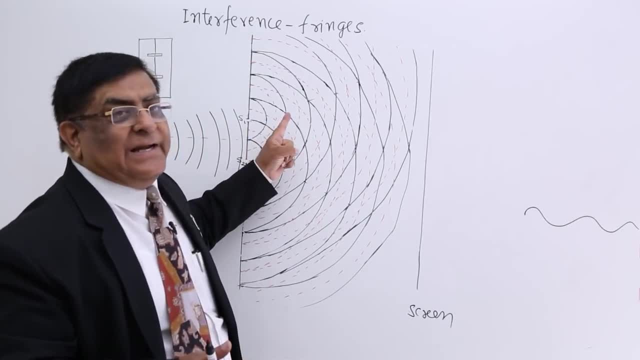 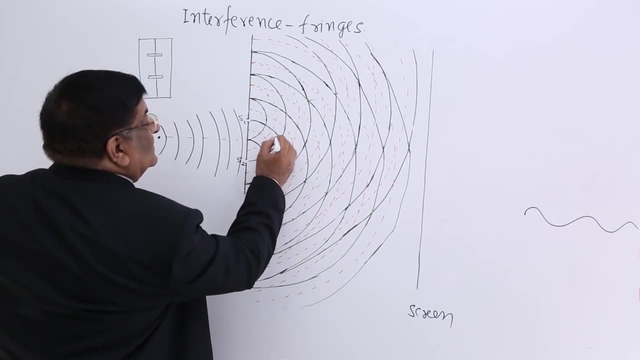 Whenever they are sending crest at any one point, we will see what happens. This is a point. this: At this point, we see S1 has sent a crest. When this crest reaches here, the crest of this also reach here. So what do we get? 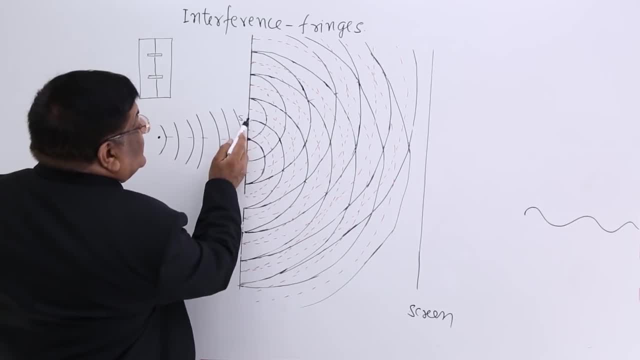 A constructive superposition. Now this S1 has sent a crest. When this crest reaches here, the crest of this also reaches here. So what do we get? S1 has sent after this crest, this one trough, and S2 has sent after this crest, this one. 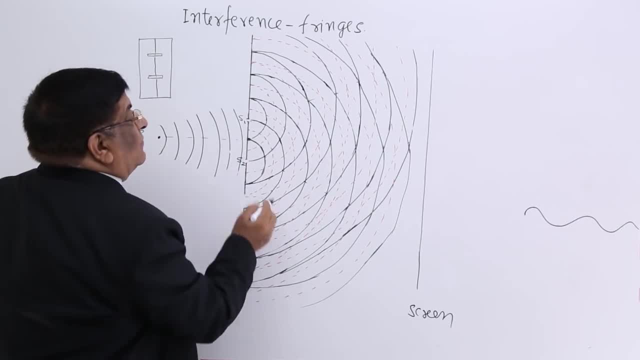 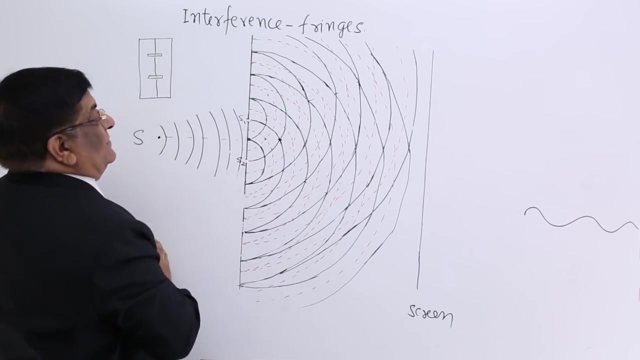 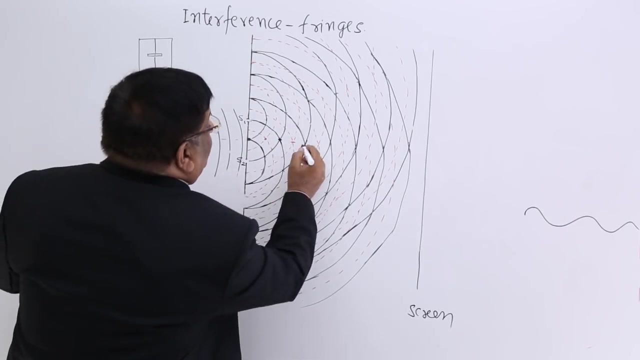 trough. Both trough meet here. What do we get here? We get here a double trough which is minus 2a. this Here, this is the second crest For this, this is the second crest. So we get a plus 2a amplitude here, then next its trough. its trough minus 2a, then plus. 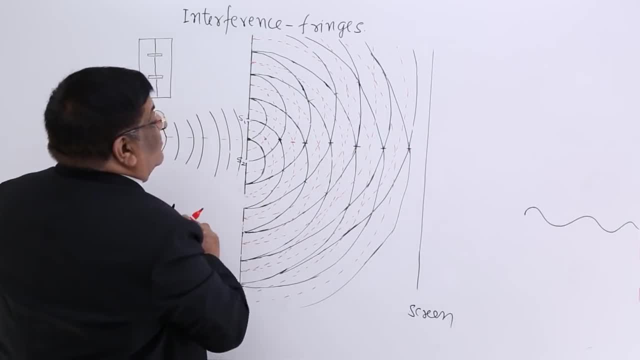 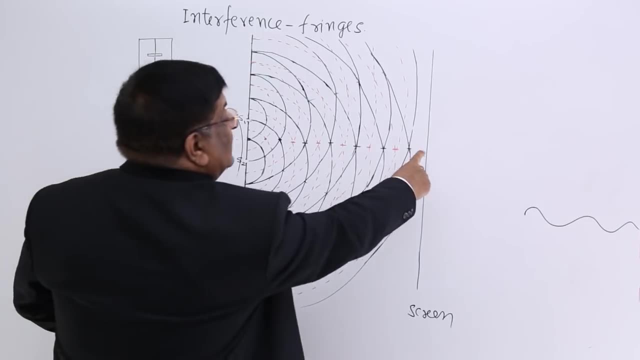 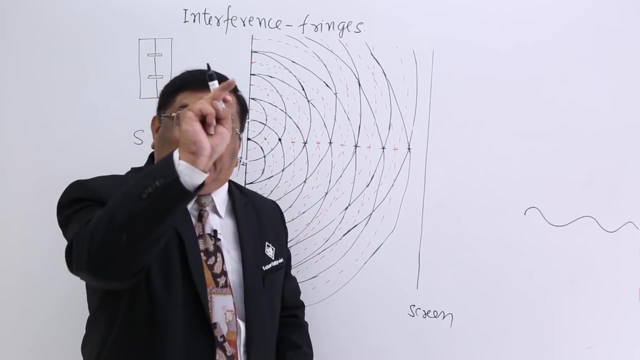 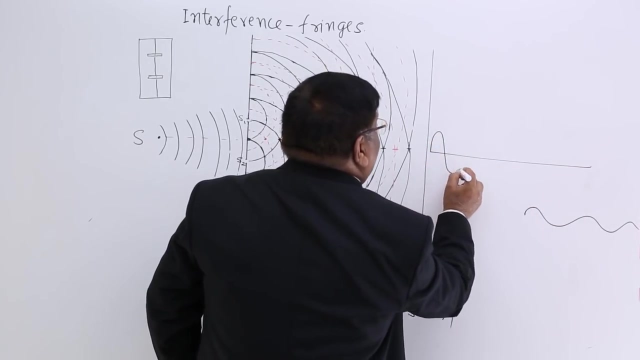 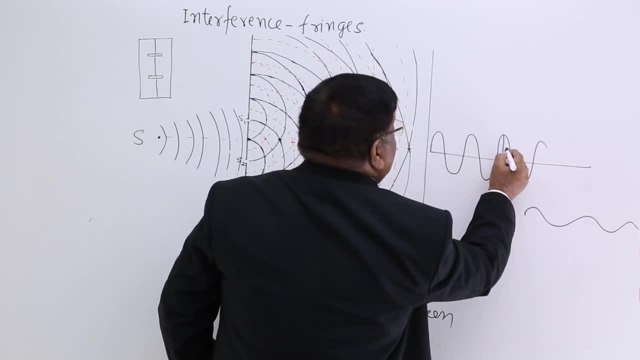 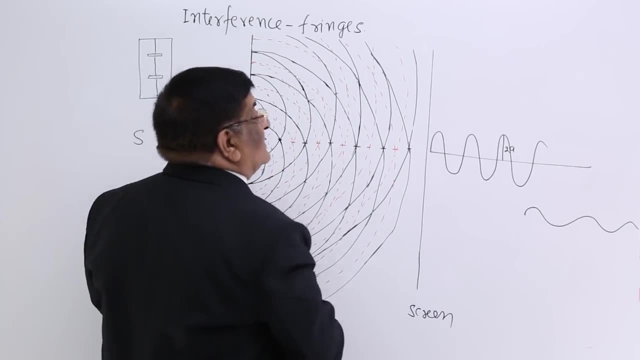 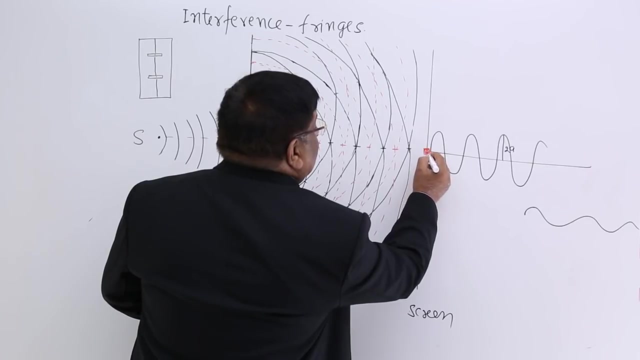 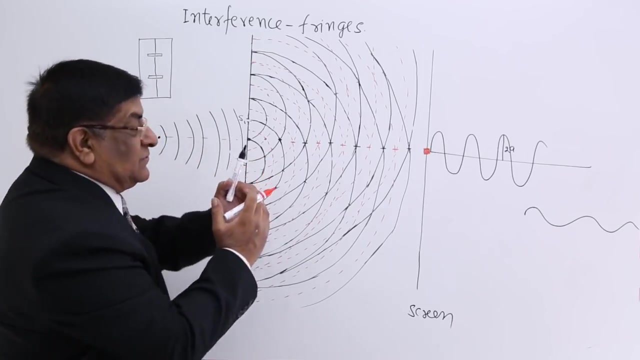 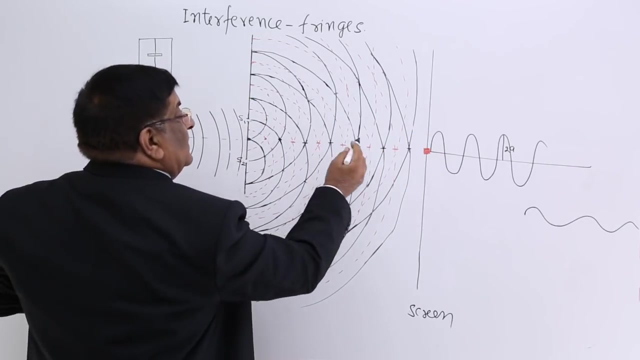 this: How much is this 2a? If this is 2a amplitude, then what is intensity? The intensity is very bright, Very bright intensity here. Now I will show you another point. The wave is going circular. This wave front will also strike this Now, this wave front, when it. 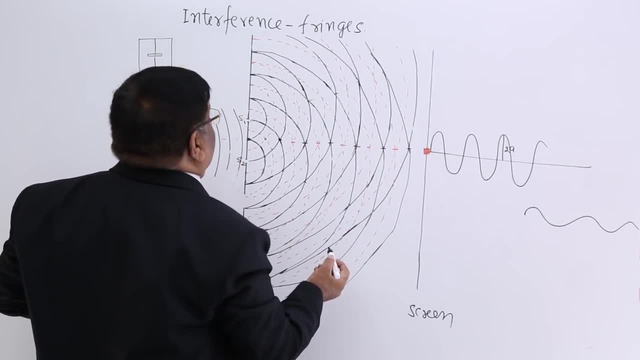 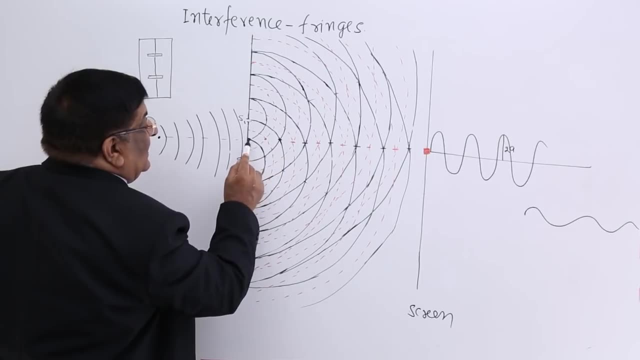 strikes at a different point. where is that different point, That different point C? This is sending a crest and this source has sent a trough. that crest and the trough, this point. At this point, what is happening? The crest by source 2 and the trough of source 1 wave here, and when crest and trough, they superpose, what do we get? 0. 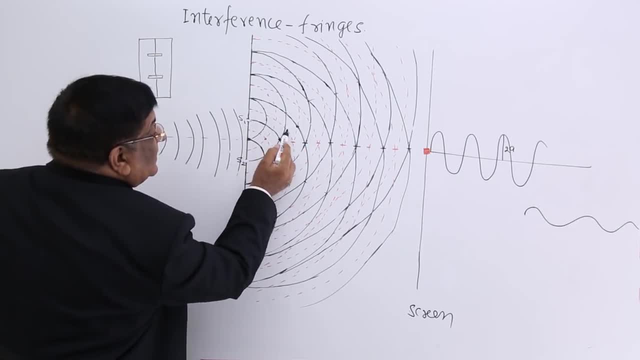 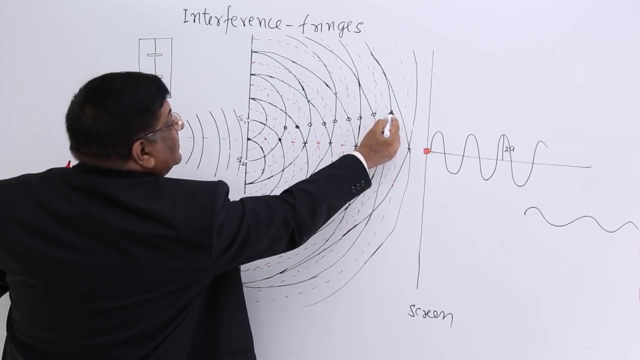 Here: this is trough, sent by source 2, this is crest, sent by source 1, 0, 0.. Here, trough, source 2, crest source 1, 0, 0, 0, 0, 0, and this way: here 0. 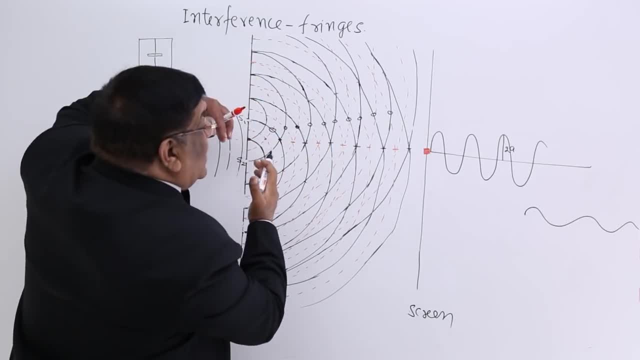 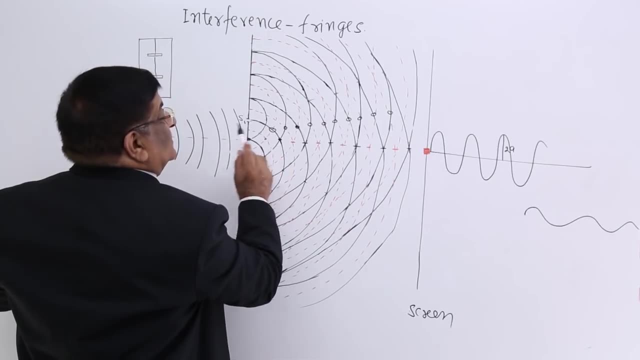 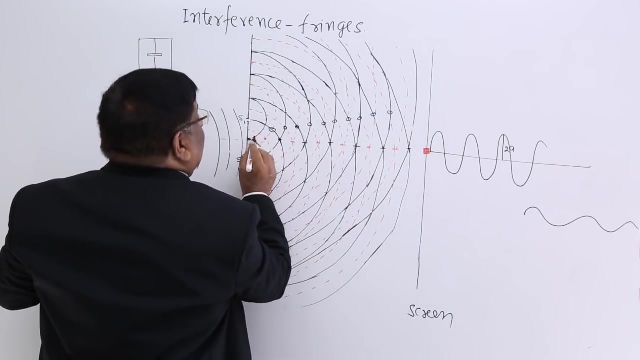 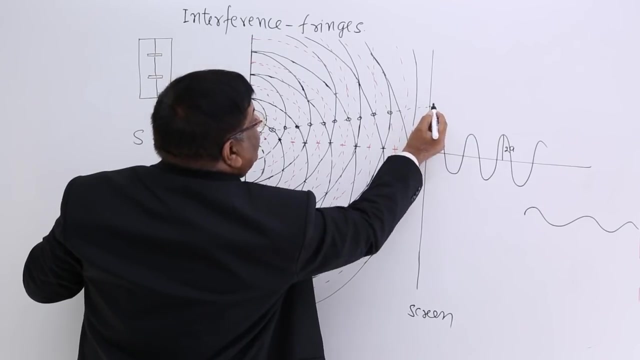 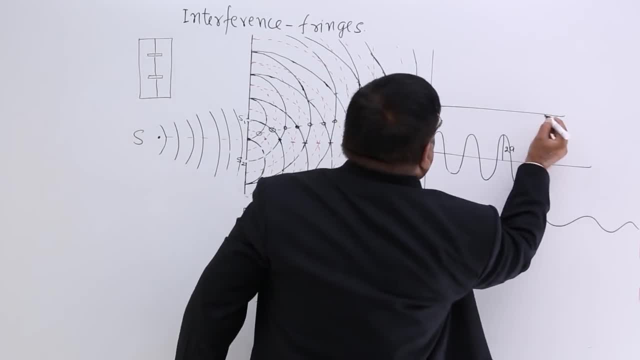 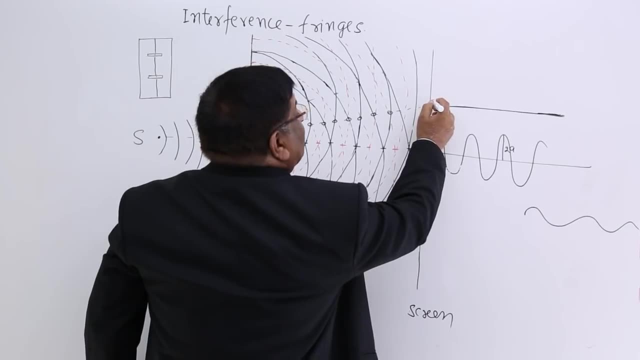 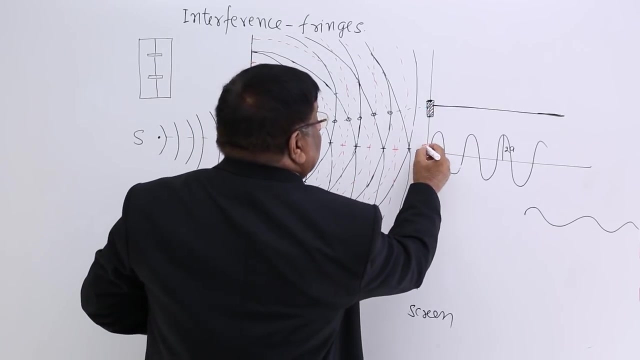 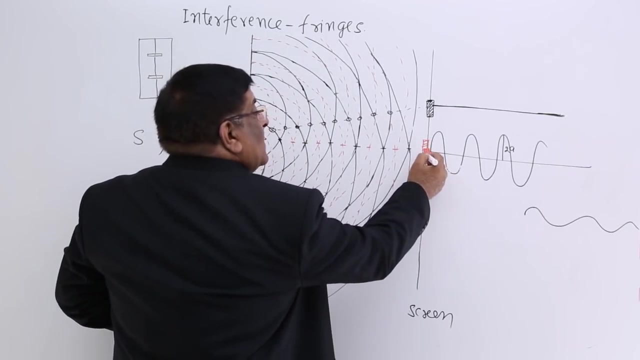 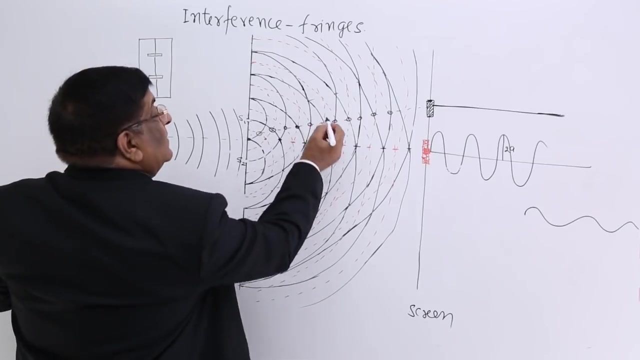 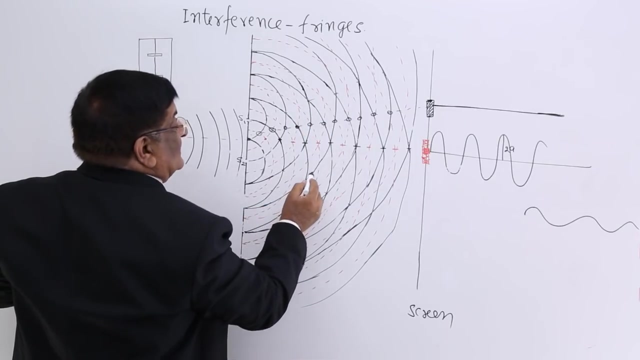 So I get no amplitude here and here. what is the wave? Simple like this: No amplitude at all. and this point is dark point, While this was a bright point. Okay, next, what will happen? Will it remain dark? Let us see Now. if I move another angle- and this angle, I find this is crest by source number 2.. 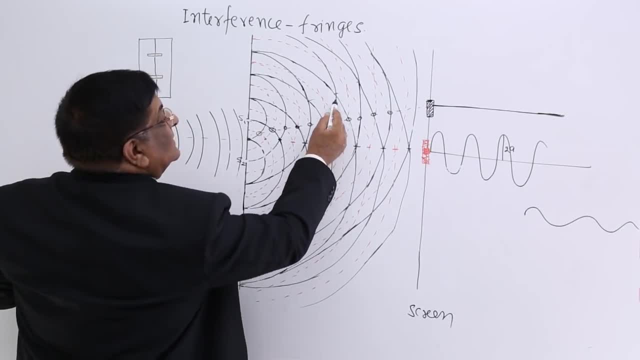 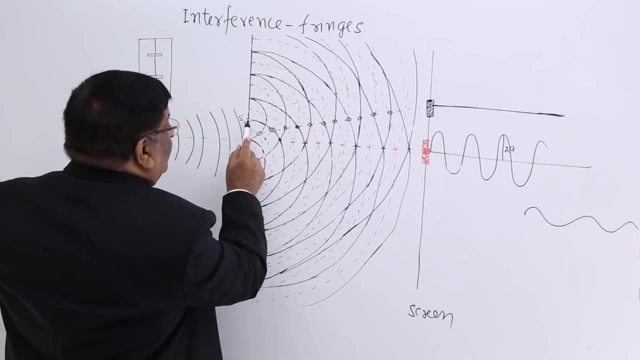 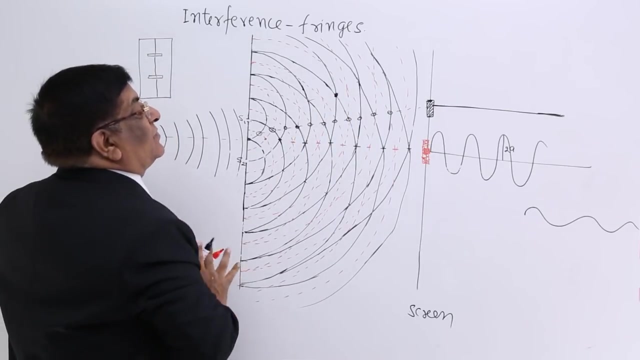 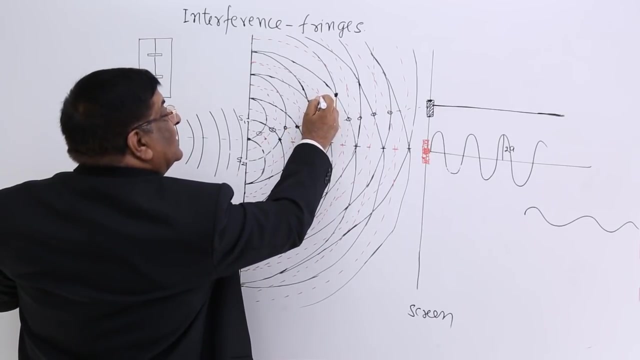 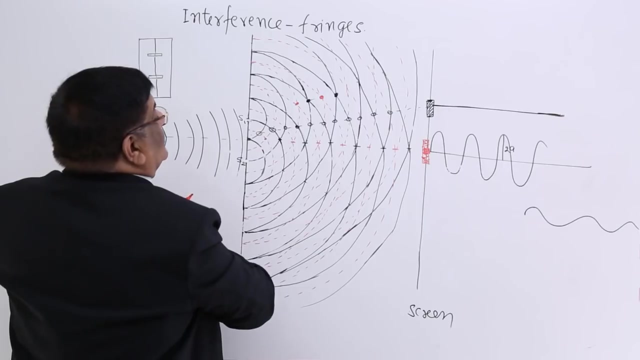 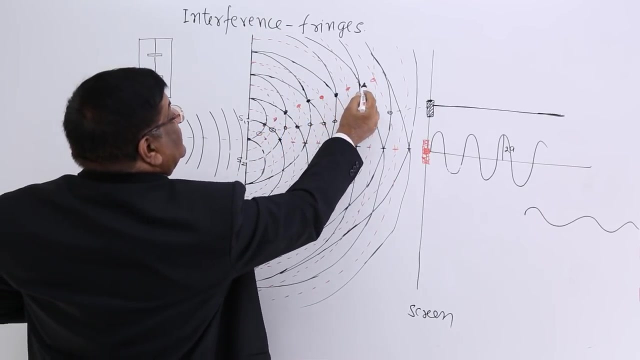 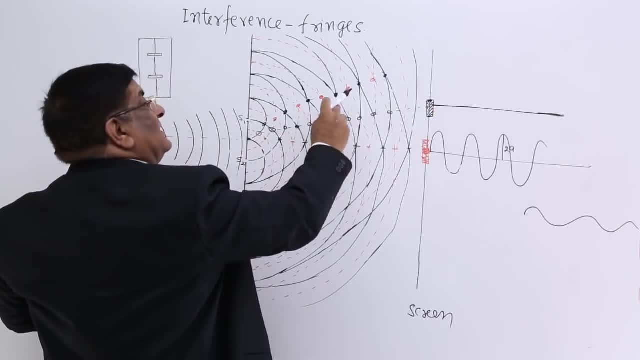 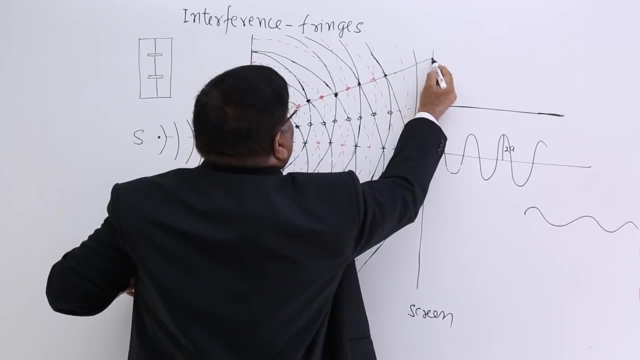 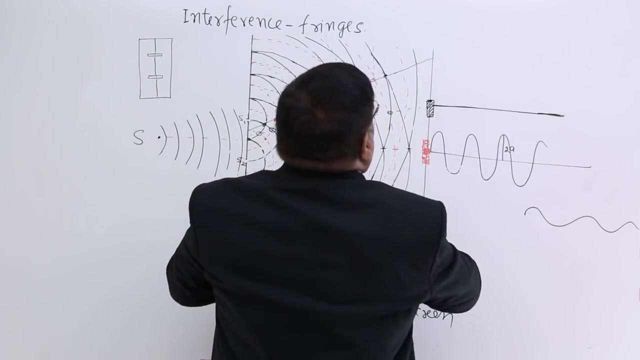 And finally, when this is the spreading wave, so this spreads this way and strike here. what do we get there? we get there amplitude 2a. so here we get an amplitude which is again 2a. so this becomes a bright point. 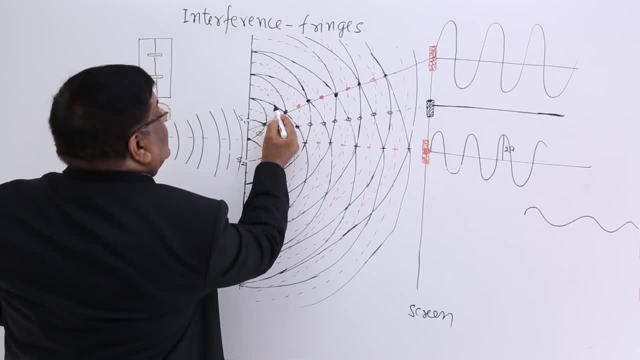 above that, here this crest, source 1 to trough off source 2, crest and trough. this point is 0 amplitude, Again 0 amplitude. after that, when we go further, it is again 0 amplitude, we get 0 amplitude. 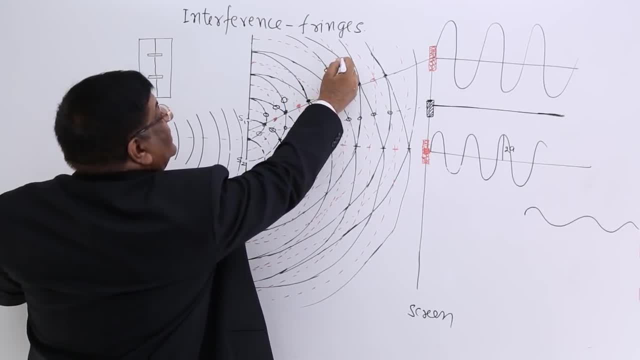 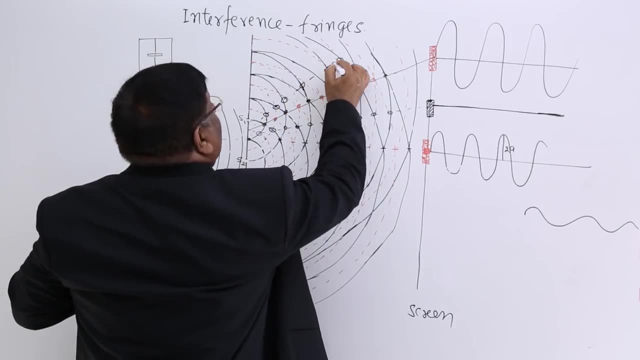 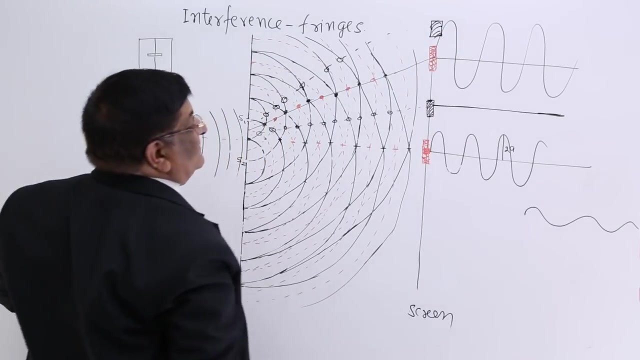 at this: 0 amplitude, 0 amplitude. if we make it uniformly, we will get 0 amplitude, like this. and when the wave is spreading, then at this point we get 0 amplitude, once again, blank. Now, when we come down, this is 0 amplitude, 0 amplitude, 0, 0. here it is 0, crest by: 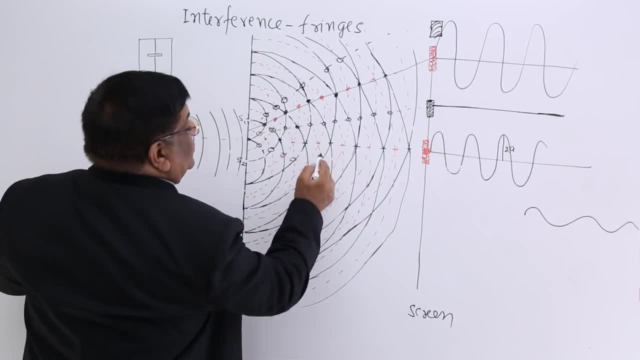 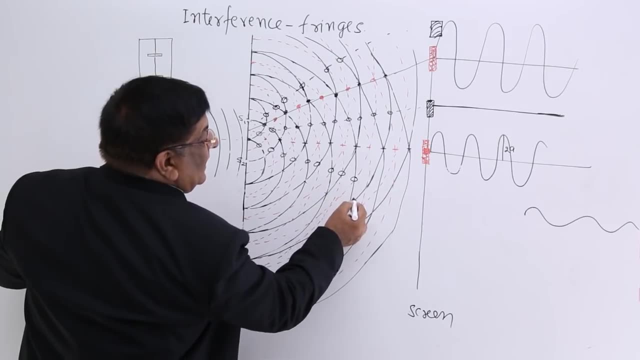 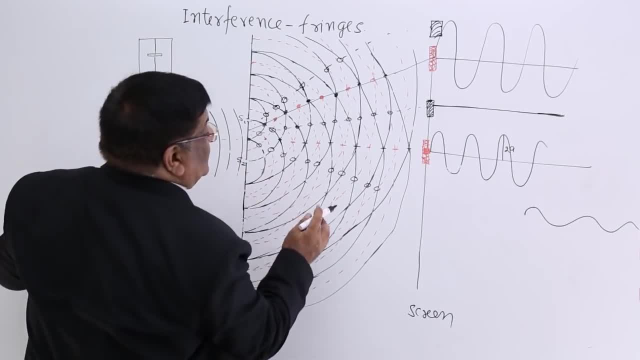 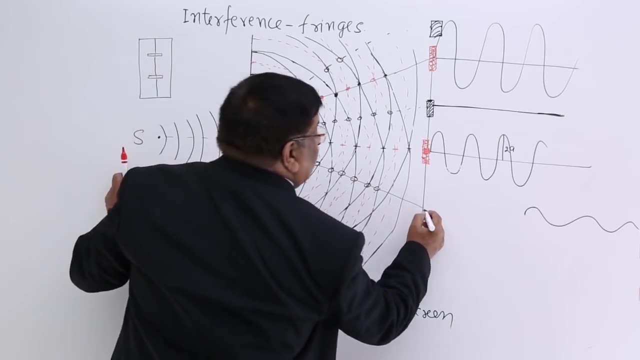 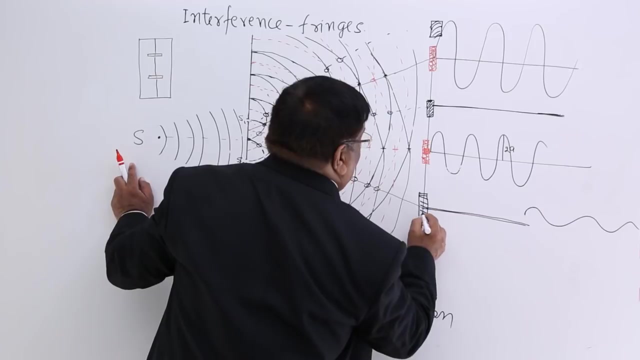 0, 0, 0, red and black: 0 and black: 0. 0, 0.. So what we get When the wave spread, there is no activity here in this direction, and here we get no activity plane, and this becomes a dark point, Dark, dark. which shape. 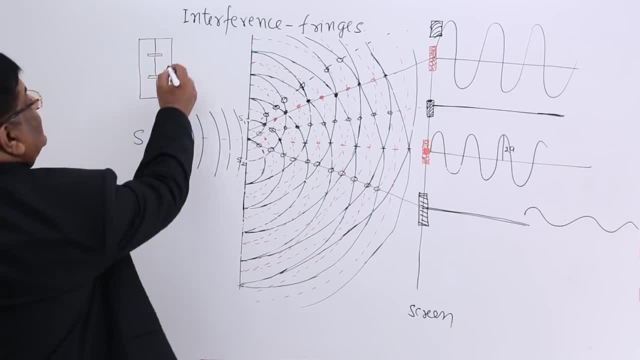 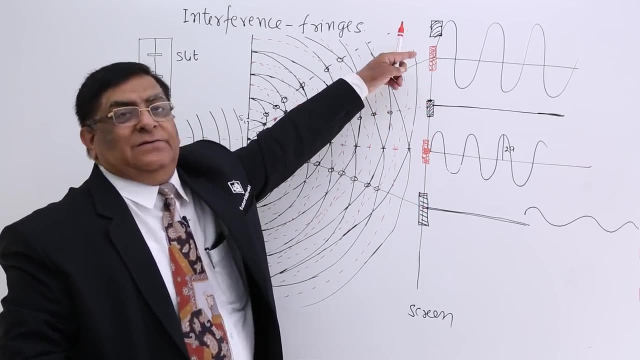 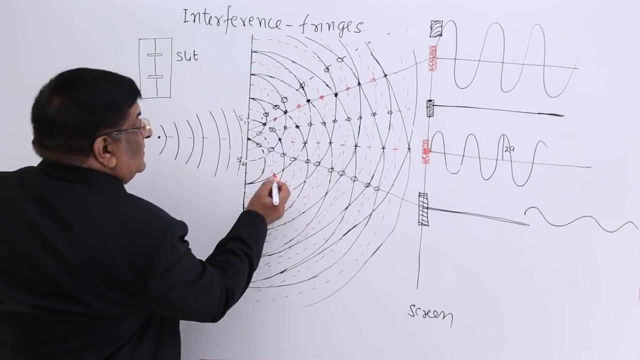 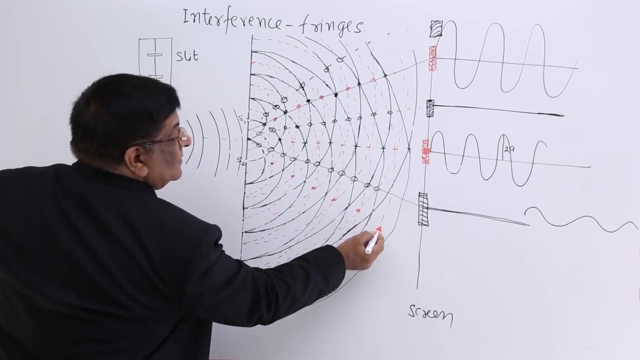 Whatever is the shape of opening, what is that Slit? So what we get here is bright slit, dark slit, dark slit, bright slit, dark slit. Here we get dark slit. Now, below that, what is happening? See again, this is trough on trough and this is crest on crest, crest. 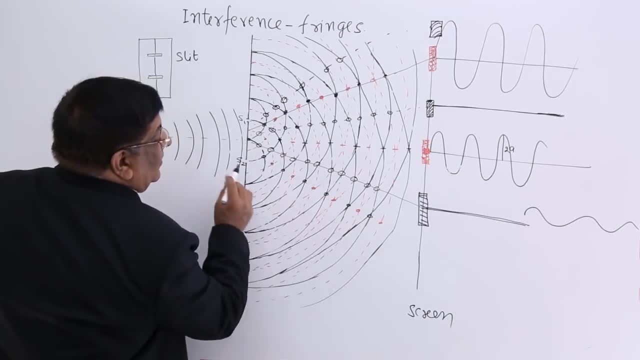 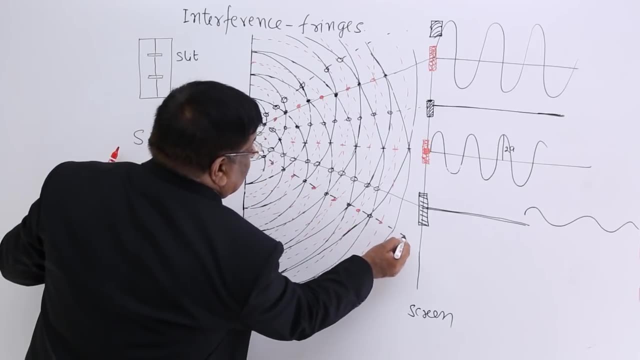 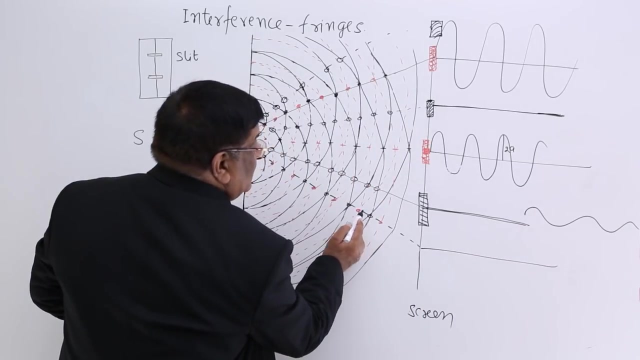 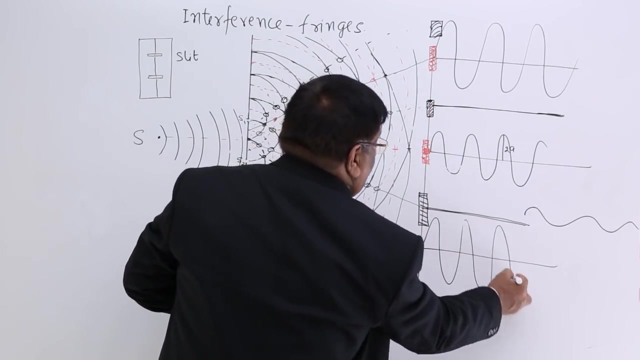 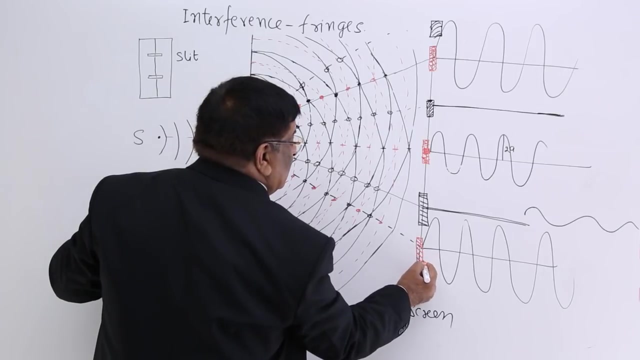 by one wave and crest by the second source, and all these are in one line spreading. So spread, they reach this point and this point. what is the wave, double crest, double trough, and it will be again like this double, and what we get here is a bright slit. so this: 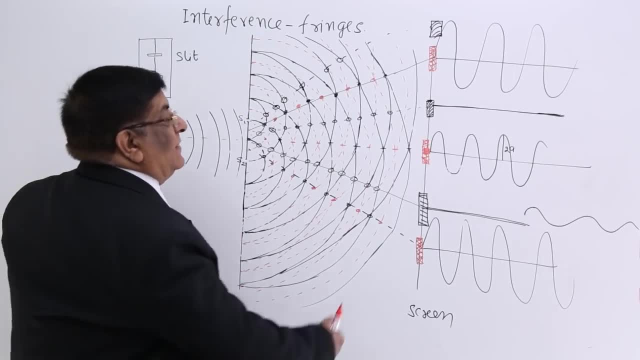 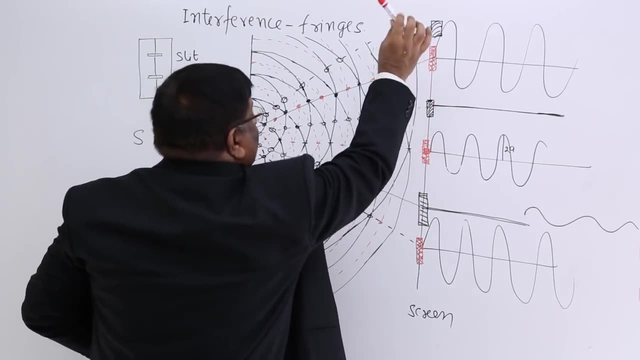 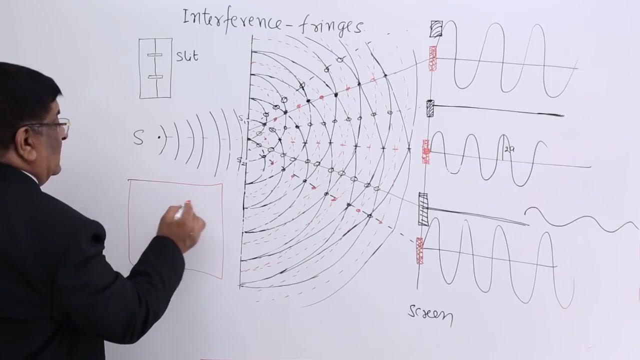 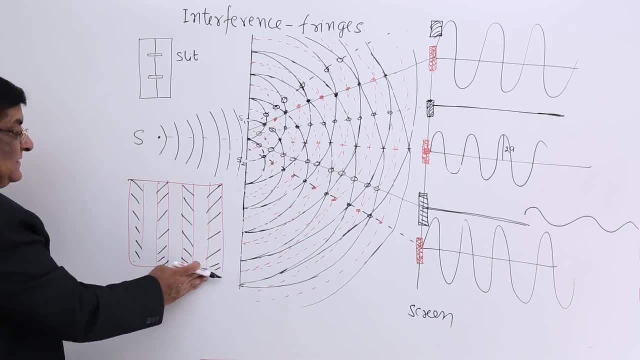 this is bright, this is dark. So this is this. pattern of the slits is known as interference pattern: bright, dark. at this point, how much is the intensity of light? 0,. at this point, how much is the intensity of light? 4 a square. 4 a square. that is intensity which is 4 times of the intensity. 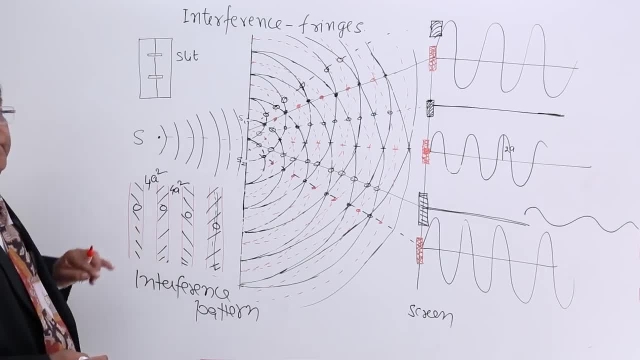 of this wave. here it is 0 times. If we would have sent one wave only, the intensity would have been a square. If we would have sent only second wave, intensity would have been 0.. If we send both, then for the two source, two sources, how much it should be a square? 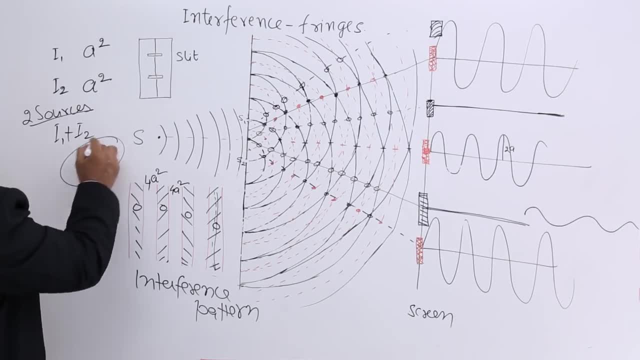 plus a square, 2 a square, but it is not 2 a square. What do we find? it is either 0 or 4 a square. How it has become 2 a square to 4 a square because of interference. 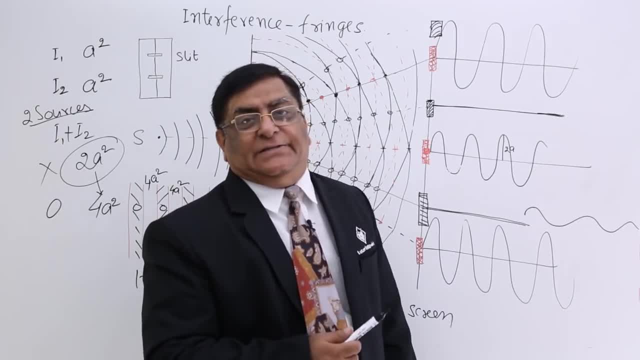 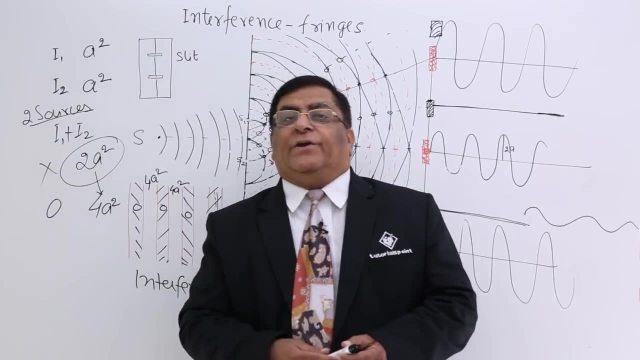 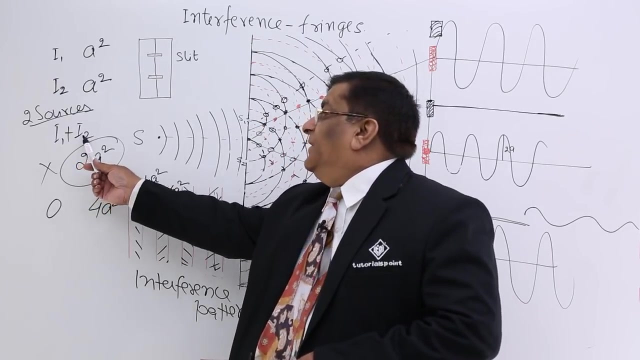 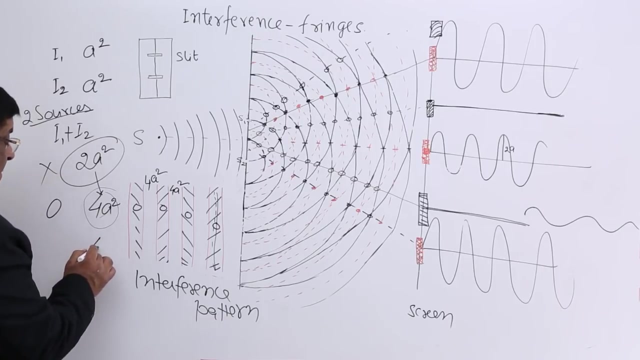 Which interference? That is constructive interference. So this is how interference takes place. sometimes it is asked from us: according to conservation of energy. we cannot increase energy, we can only transfer it. So how this combination has given us so much 4 times of energy, that is 4i- why. 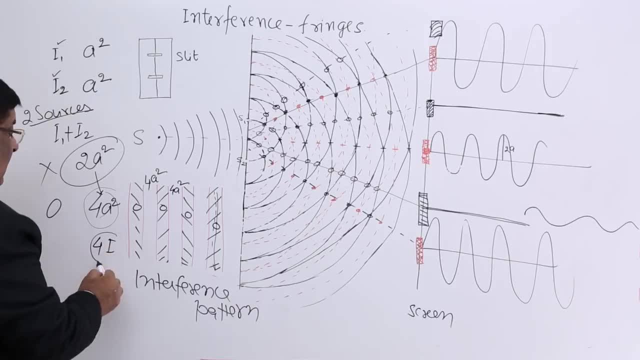 This is 1i. this is 1i intensity. how it has become 4i? Our answer is that here it has become 0. If you make total of all this should have 2i, 2i, 2i, 2i. 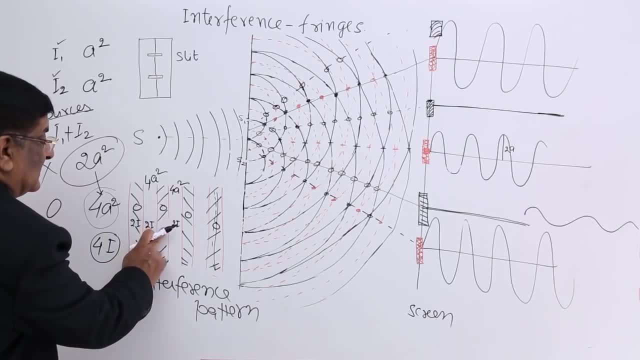 Now what has happened From this place? the intensity has become 0, that 2i is shifted here and it has become 4i. So this is a simple case of transfer. So this is a simple case of transfer. So this is a simple case of transfer. 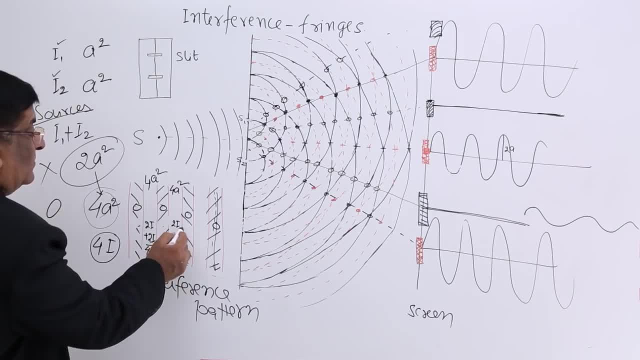 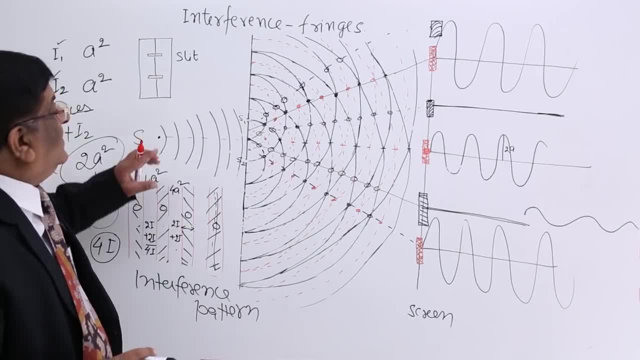 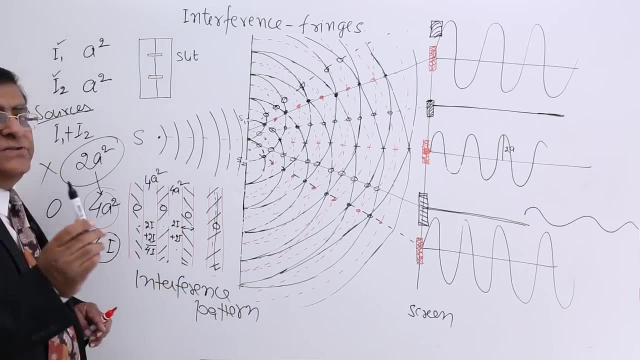 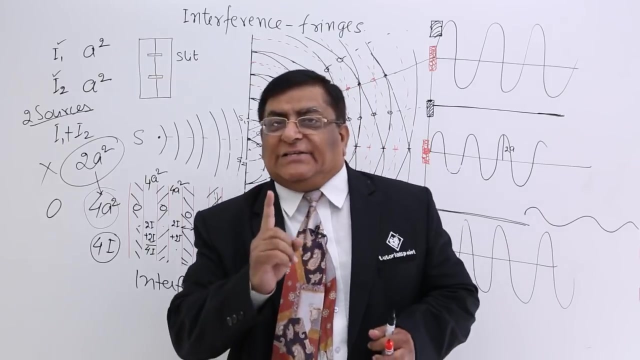 This is one thing: transfer of energy. Another thing: the interference pattern. there are no clear cut lines like this. this we have made just to make it understand, Otherwise what happens. what I am telling is a bright slits. this is very bright at. 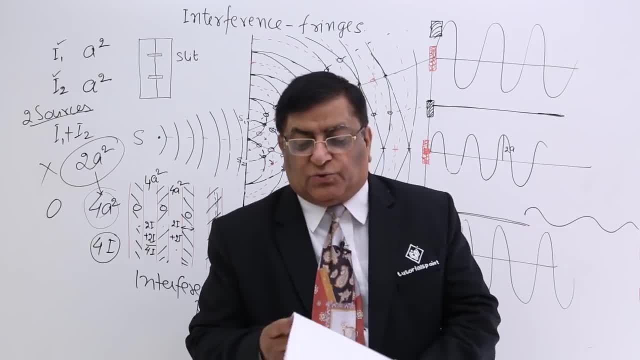 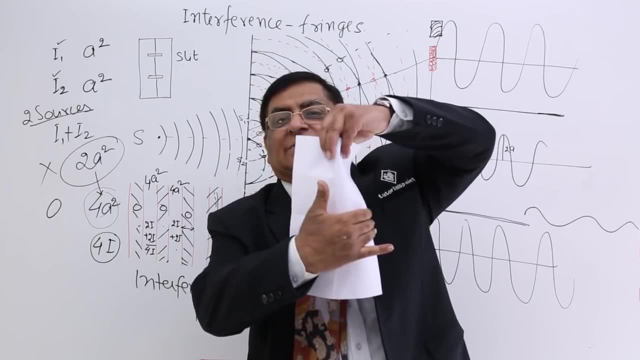 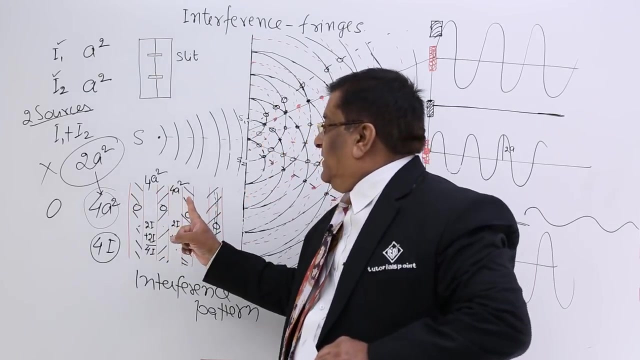 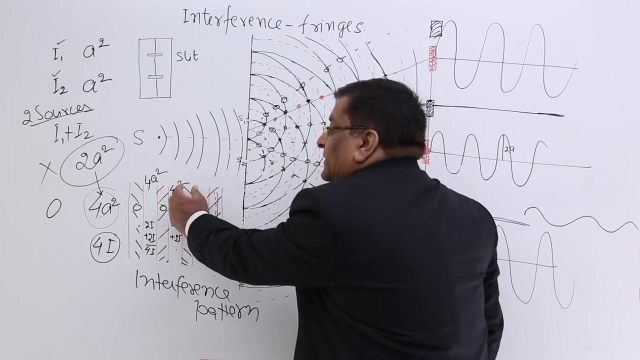 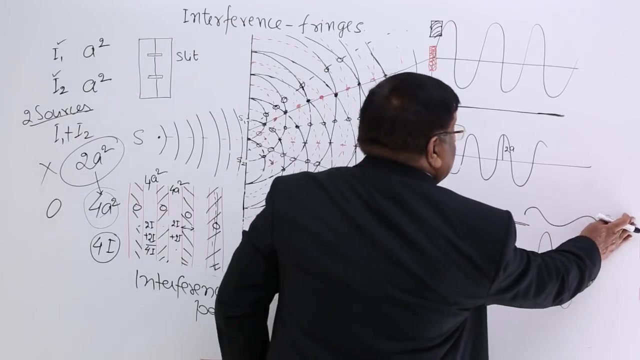 the center, but then brightness goes on decreasing. this way, bright brightness goes on decreasing, then decrease, decrease, decrease. minimum here dark. so at the dark there is a minimum darkness, but the complete darkness is not in a strip, not in a strip. this is simply like this. i will show here that this is dark, very dark, and this darkness goes on decreasing. it is 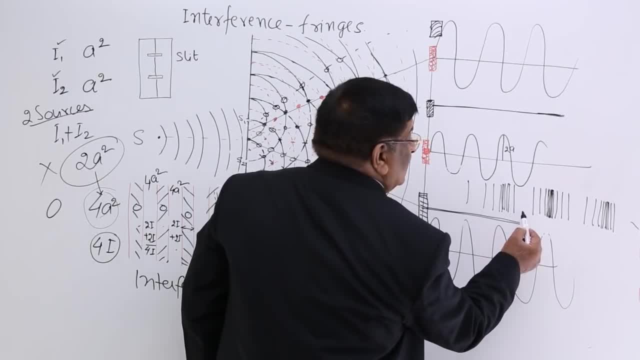 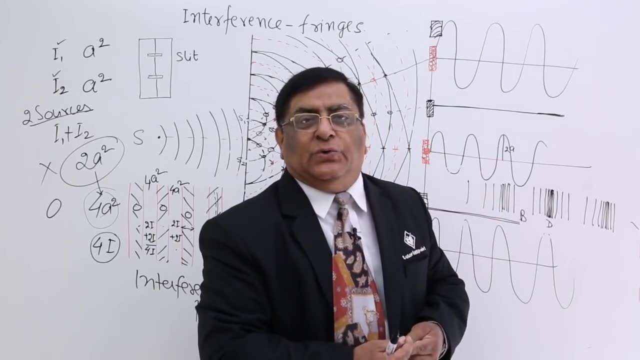 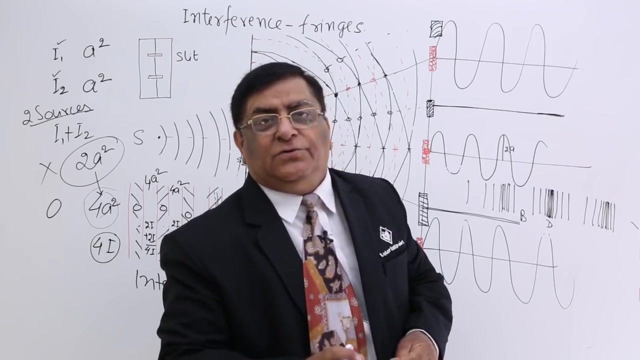 like this: this is the brightest spot and this is the darkest spot. there is no clear light, clear cut line between them. so we have found a method to find out the width. how do we measure the width? if i want to find out width of a dark fringe, i will see the brightest point. 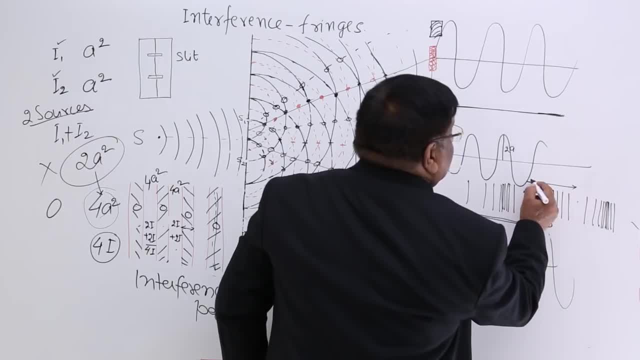 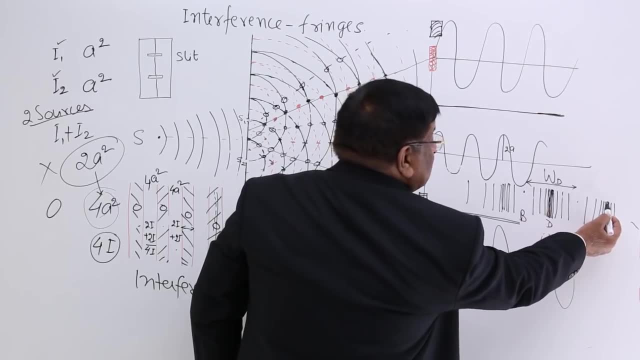 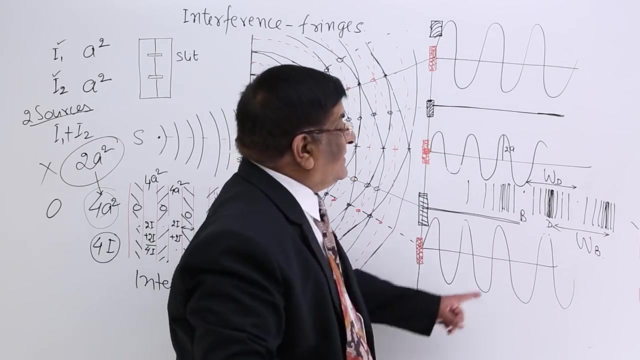 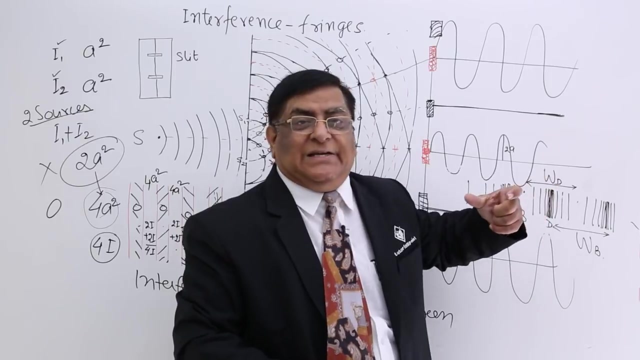 and the next brightest point. this width is known as width of the dark fringe, and this is a darkest point. this is the darkest point. this width is known as width of the bright fringe. so what is width of the bright fringe? it is the distance between the two dark most point, adjacent dark most point. what is the width of the dark fringe? 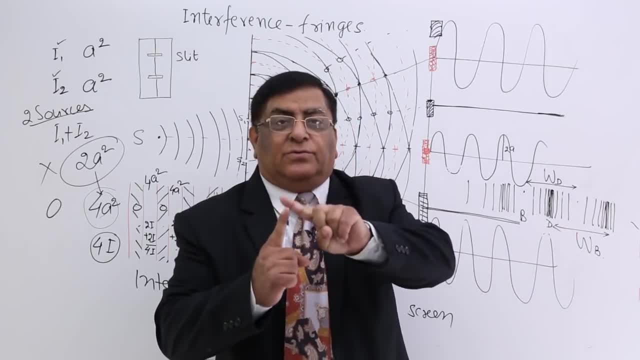 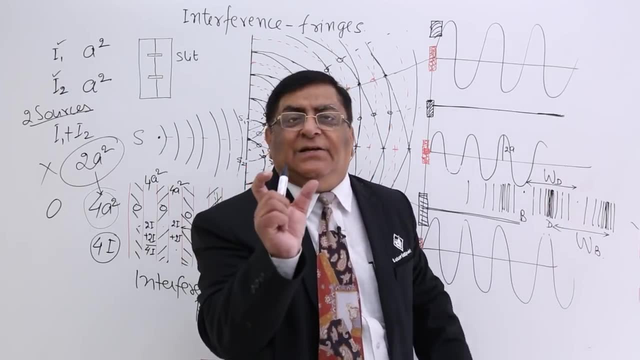 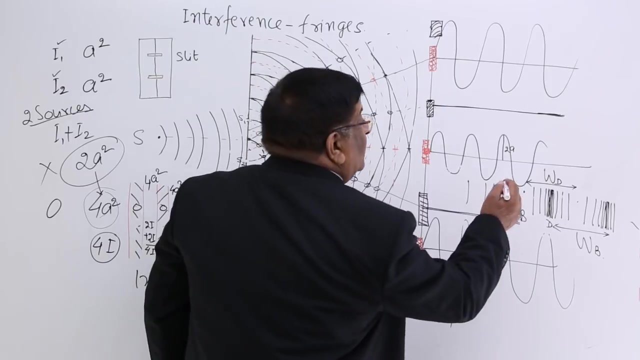 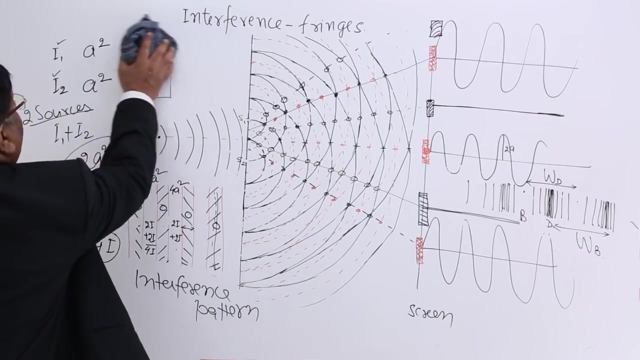 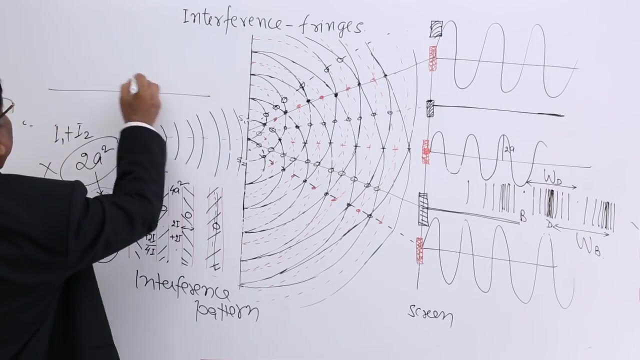 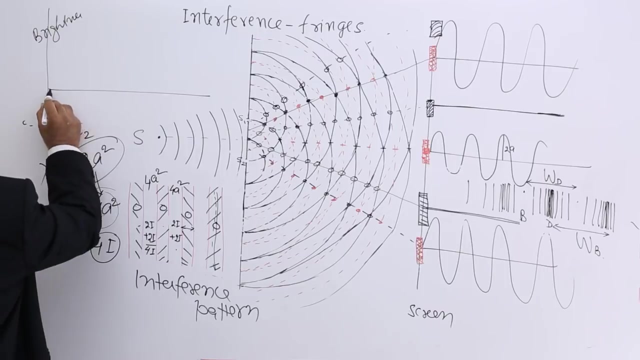 it is the distance between two. next these are: these are two bright fringes, adjacent bright fringes. the distance between them is the width of dark fringe. so if we make a graph of this, the graph, and that is a famous interference graph, if i show the brightness by y axis brightness and this is the distance, this is center point. 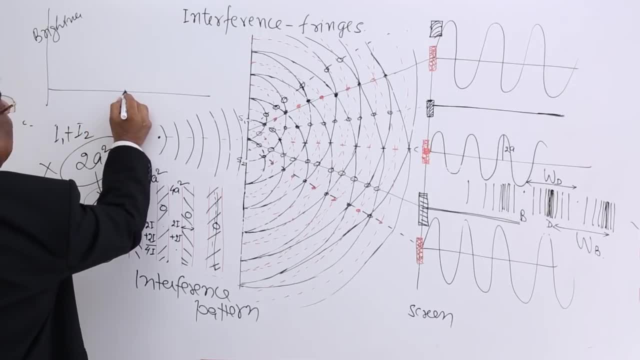 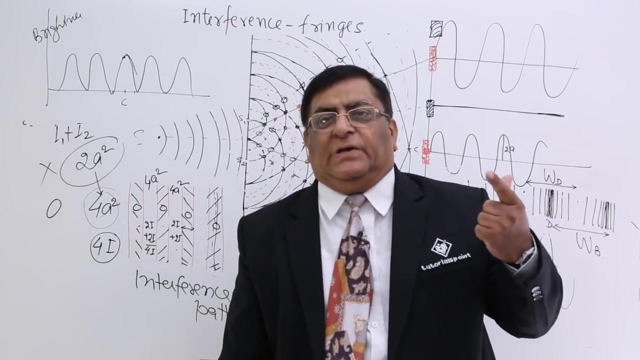 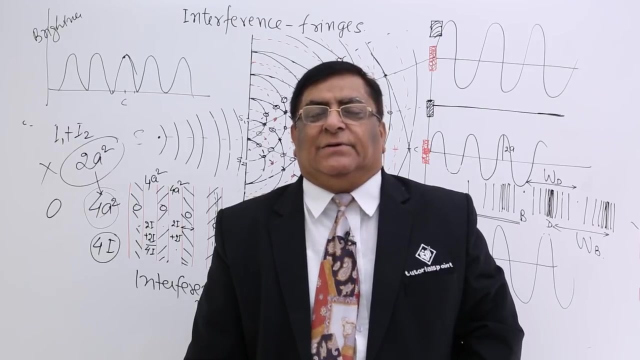 c, c, then at c the brightness is maximum, then at this distance it will become less and we get a graph like this. okay, we will make it again when we do the next experiment. but this was theory put forward by eisen. he said these fringes will be formed like this, then there. 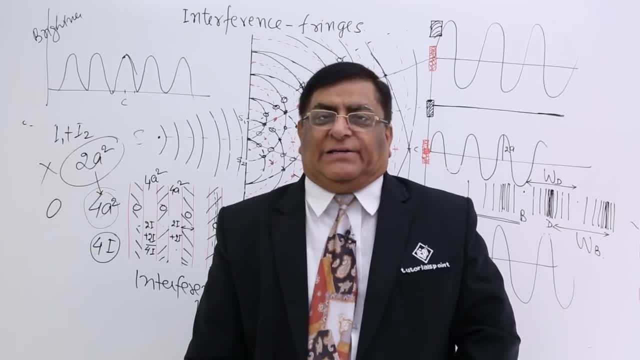 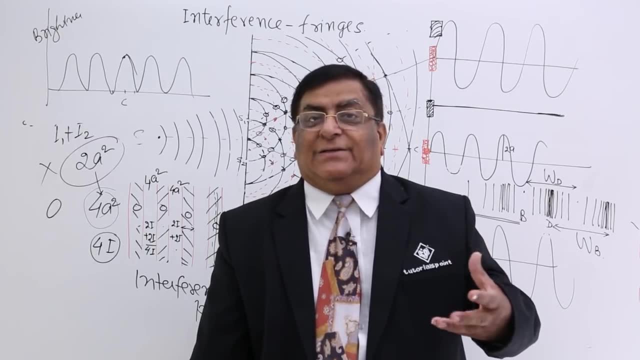 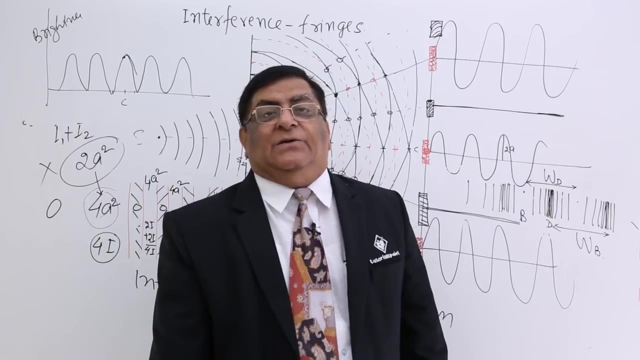 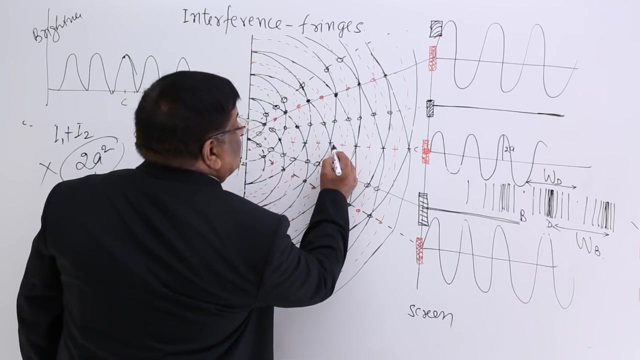 was lot of obviousness, that it is easy to write it on the paper, to make it theoretically and to calculate all the things, what things? what will be the width of the fringe calculated? how the fringes are related with wavelength, that is calculated. so, all these, what is wavelength, this distance? this is the wavelength.